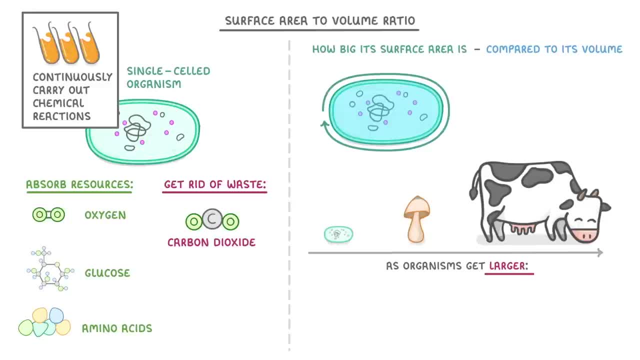 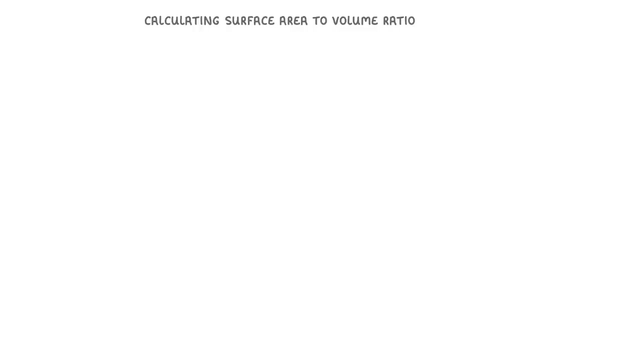 organisms get larger- for example, comparing this single bacterial cell to a mushroom or a cow- their surface area to volume ratio decreases, Which is just the technical way of saying that larger organisms have less surface area compared to their volume. Now calculating the surface area and volume of a real organism is actually really hard. 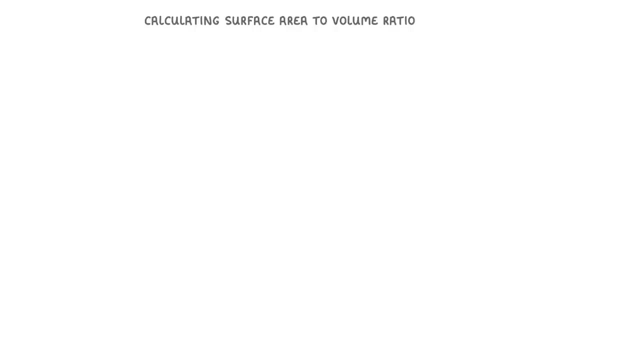 because they're weird shapes. So instead, to see this idea in practice, let's take these three cubes and see how their surface area to volume ratio changes as they get bigger. To calculate the surface area of a cube, you just calculate the area of a single face. 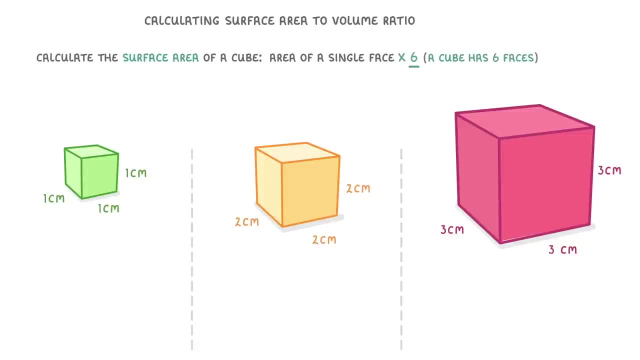 and then multiply it by six, because a cube has six faces. So we get the area of one face by doing one centimetre times one centimetre, which is just one square centimetre, And then we multiply it by six to get a total surface area of. 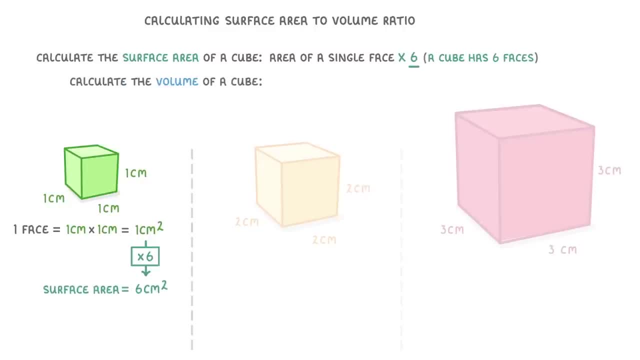 six square centimetres. Then to calculate the volume of a cube, we just multiply the length, width and height together. So for our green cube that's a volume of one centimetre times one centimetre, so one cubic centimetre, And so the surface area to volume ratio is 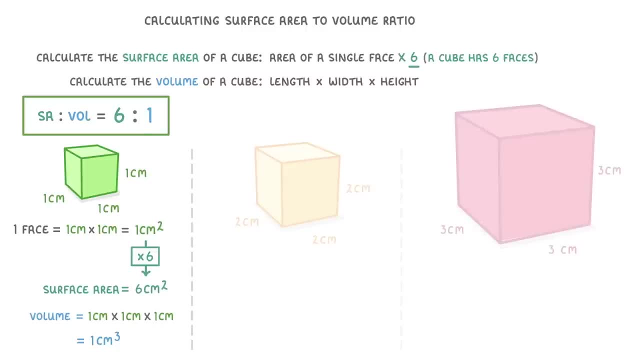 just the surface area of six to the volume of one, Which basically just means that the surface area is six times bigger than the volume. If we do the same thing for this medium cube, though, we get a surface area of 24 square centimetres and a volume of eight cubic centimetres. 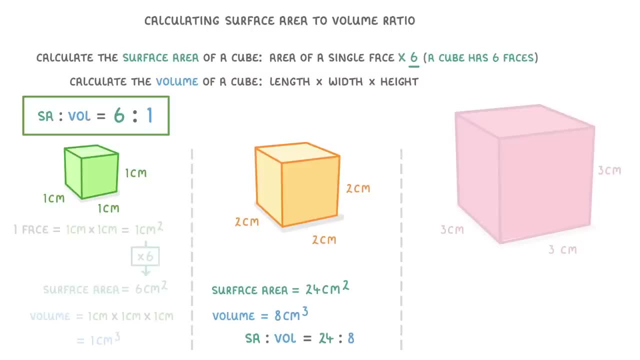 And so a ratio of 24 to eight, which simplifies to three to one. And if we do the same thing for the biggest cube, we get a surface area of 54,, a volume of 27, and a ratio of two to one. So if we now compare the smallest and biggest cubes, we can see that as the 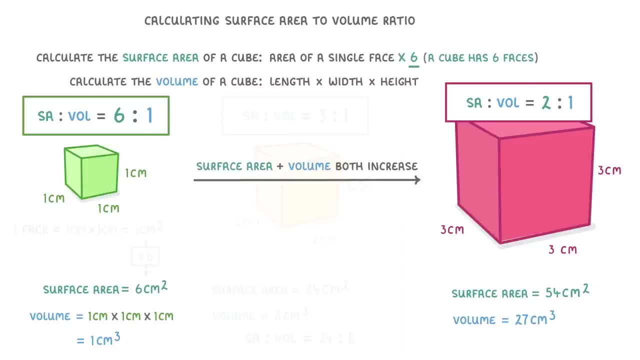 cubes get larger. their surface area and their volume both increase, But, importantly, their volume increases much more quickly. For example, the surface area only gets nine times larger here, but the volume gets 27 times larger, And this is why the surface area to volume. 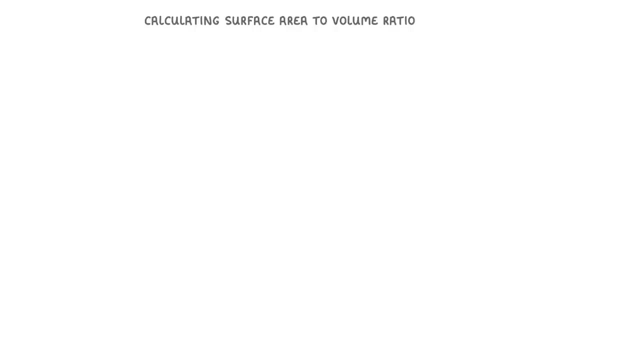 because they're weird shapes. So instead, to see this idea in practice, let's take these three cubes and see how their surface area to volume ratio changes as they get bigger. To calculate the surface area of a cube, you just calculate the area of a single face. 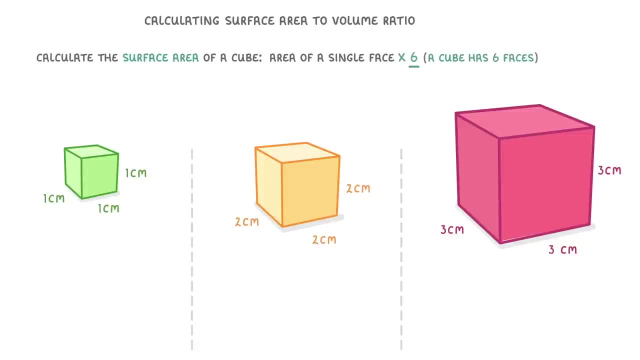 and then multiply it by six, because a cube has six faces. So we get the area of one face by doing one centimetre times one centimetre, which is just one square centimetre, And then we multiply it by six to get a total surface area of. 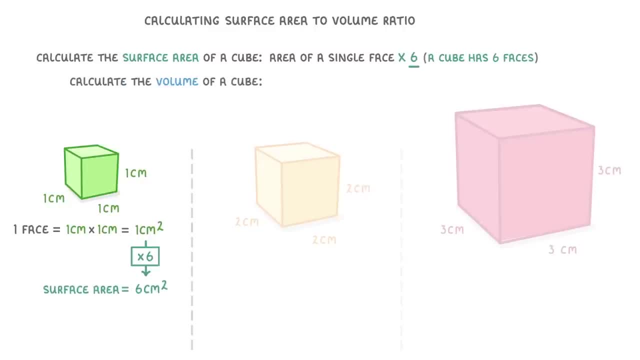 six square centimetres. Then to calculate the volume of a cube, we just multiply the length, width and height together. So for our green cube that's a volume of one centimetre times one centimetre, so one cubic centimetre, And so the surface area to volume ratio is 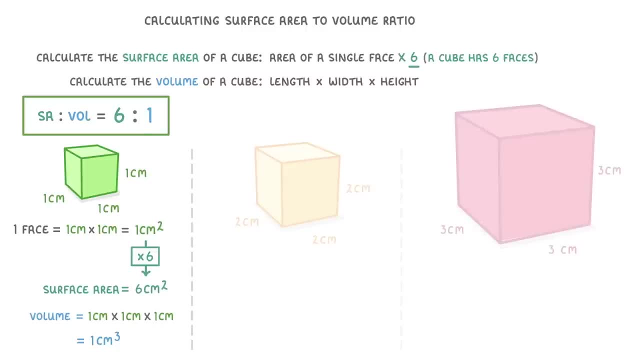 just the surface area of six to the volume of one, Which basically just means that the surface area is six times bigger than the volume. If we do the same thing for this medium cube, though, we get a surface area of 24 square centimetres and a volume of eight cubic centimetres. 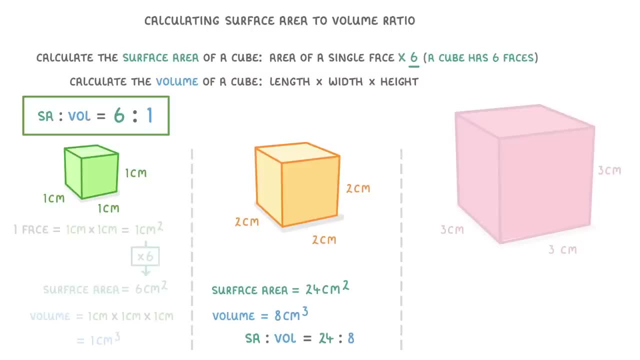 And so a ratio of 24 to eight, which simplifies to three to one. And if we do the same thing for the biggest cube, we get a surface area of 54,, a volume of 27, and a ratio of two to one. So if we now compare the smallest and biggest cubes, we can see that as the 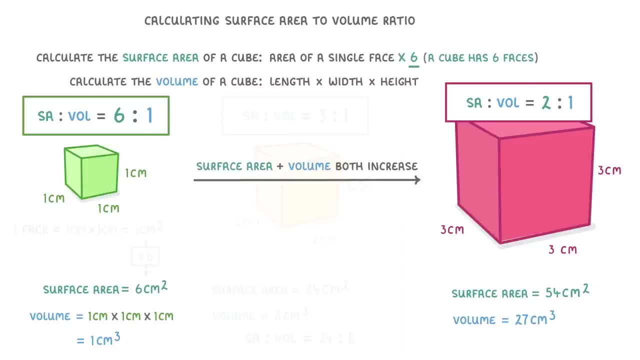 cubes get larger. their surface area and their volume both increase, But, importantly, their volume increases much more quickly. For example, the surface area only gets nine times larger here, but the volume gets 27 times larger, And this is why the surface area to volume. 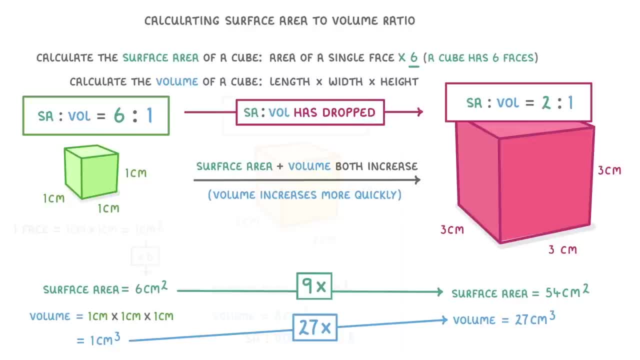 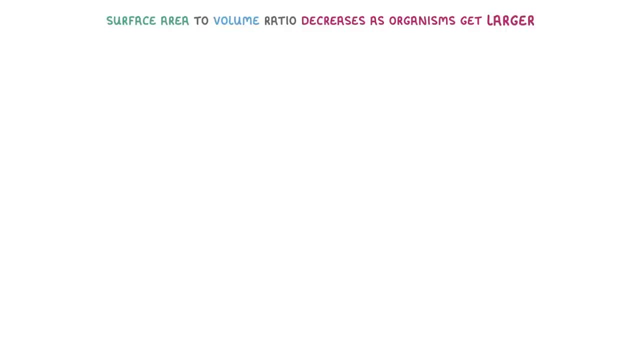 ratio has dropped from six to one to two to one. So now that you understand why the surface area to volume ratio decreases as organisms get larger, let's apply that knowledge to bacteria and humans. Because bacteria are tiny, they have a really high surface area to volume ratio, and this 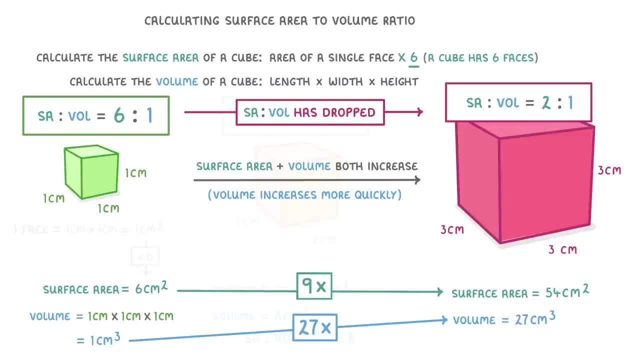 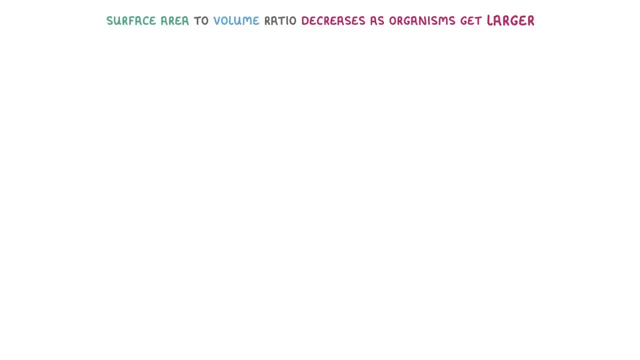 ratio has dropped from six to one to two to one. So now that you understand why the surface area to volume ratio decreases as organisms get larger, let's apply that knowledge to bacteria and humans. Since bacteria are tiny, they have a really high surface area to volume ratio, and this 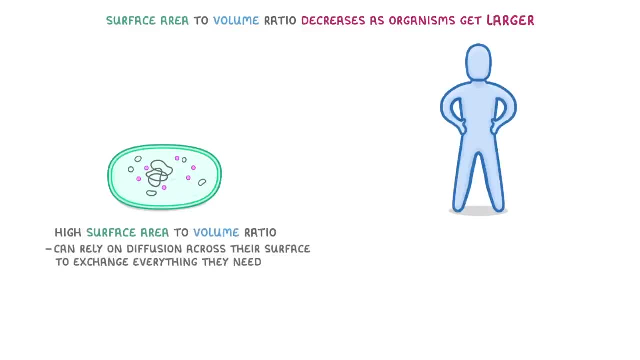 means that they can rely on diffusion across their surface to exchange everything that they need. On the other hand, because humans are so big, we have a low surface area to volume ratio, which means that we can't rely on diffusion for all of our needs Instead, 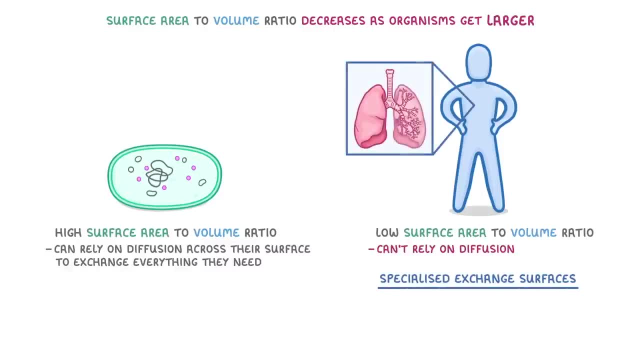 we have to have specialized exchange surfaces, like the lungs and intestines, which effectively increase our surface area to volume ratio by giving us a huge extra surface. on the insides of our body, For example in the lungs, we have millions of alveoli which together gives 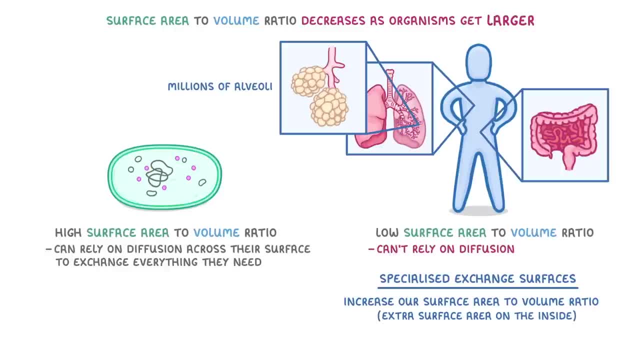 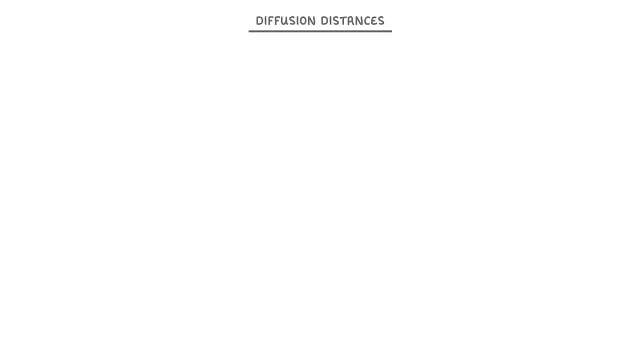 a huge surface area over which we can absorb oxygen and get rid of carbon dioxide, And in the intestines we have villi which provide a massive surface area for the absorption of nutrients. Now, another important concept to bear in mind here is diffusion distances As organisms. 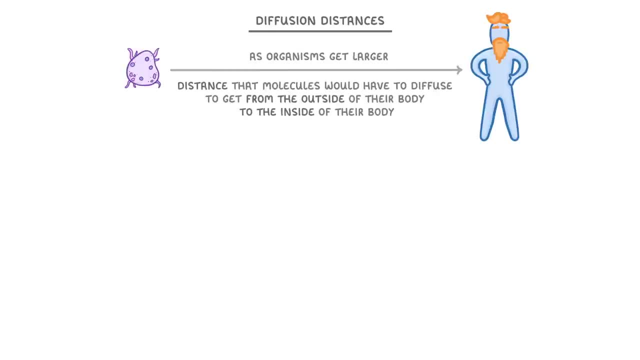 get larger, the distance that molecules would have to diffuse to get from the outside of their body to the inside of their body increases massively. For example, to get from the outside to the middle of a bacteria is probably only something like 1 micrometer, whereas to get 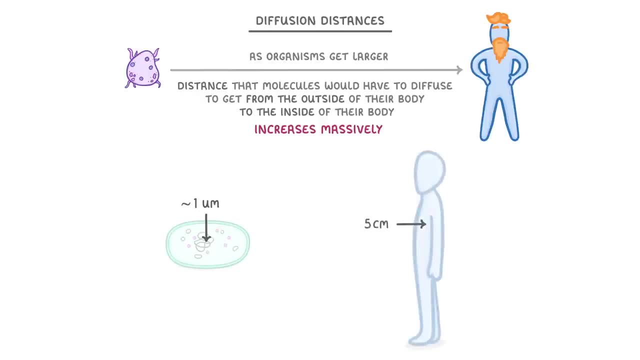 from the surface to the middle of a human would be at least 5 centimeters, which means molecules would have to diffuse 50,000 times further. This is really important, because it means that diffusion will be way slower for larger organisms, and so they won't be. 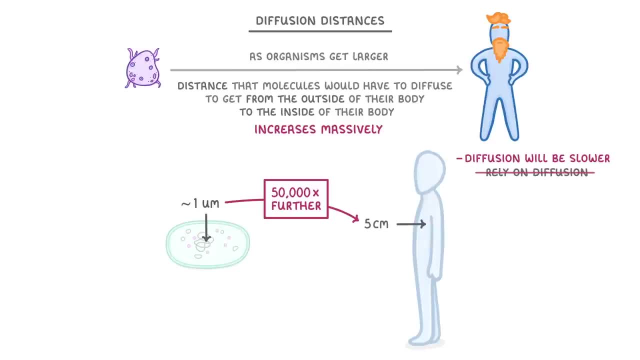 able to rely on diffusion alone to get all of the stuff that they need into their cells. To solve this, larger organisms often have transport systems, like the circulatory system, which transport molecules from the exchange surfaces where they enter the body around. 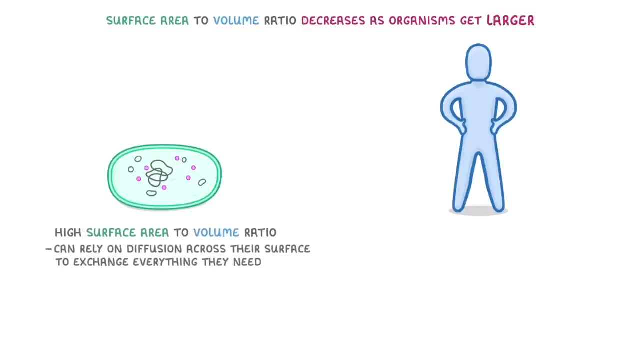 means that they can rely on diffusion across their surface to exchange everything that they need. On the other hand, because humans are so big, we have a low surface area to volume ratio, which means that we can't rely on diffusion for all of our needs Instead, 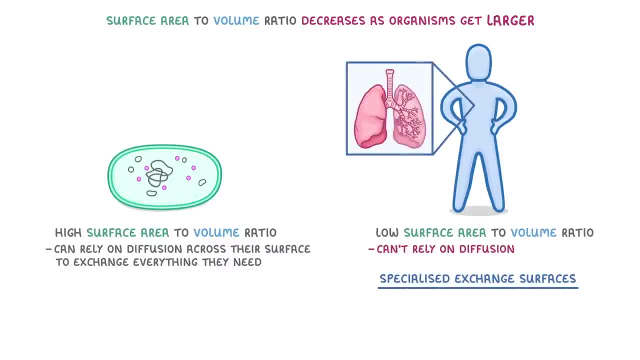 we have to have specialised exchange surfaces, like the ligands, lungs and intestines, which effectively increase our surface area to volume ratio by giving us a huge extra surface. on the insides of our body, For example in the lungs, we have millions of alveoli which together gives a huge surface. 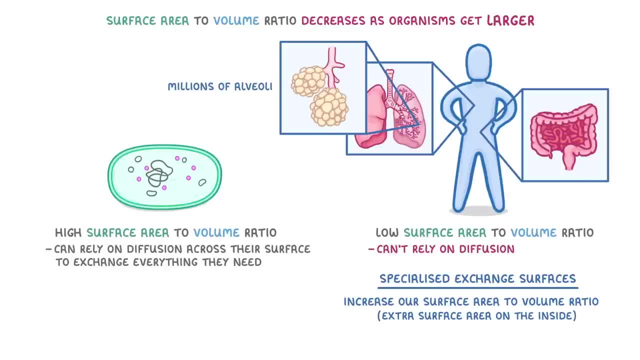 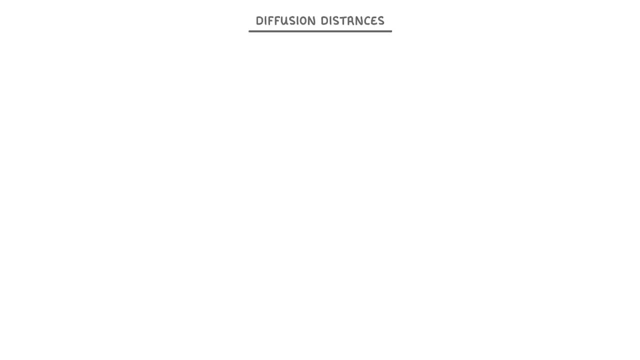 area over which we can absorb oxygen and get rid of carbon dioxide, And in the intestines we have villi which provide a massive surface area for the absorption of nutrients. Now, another important concept to bear in mind here is diffusion distances. As organisms get larger, the distance that molecules would have to diffuse to get from. 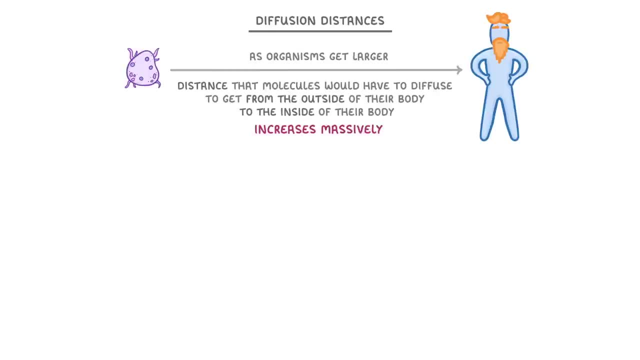 the outside of their body to the inside of their body increases massively. For example, to get from the outside to the middle of a bacteria is probably only something like 1 micrometer, whereas to get from the surface to the middle of a human would be. 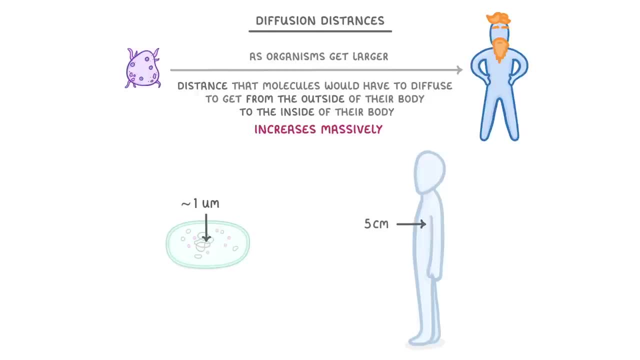 at least 5 centimeters, Which means molecules would have to diffuse 50,000 times further. This is really important, because it means that diffusion will be way slower for larger organisms, and so they won't be able to rely on diffusion alone to get all of the stuff. 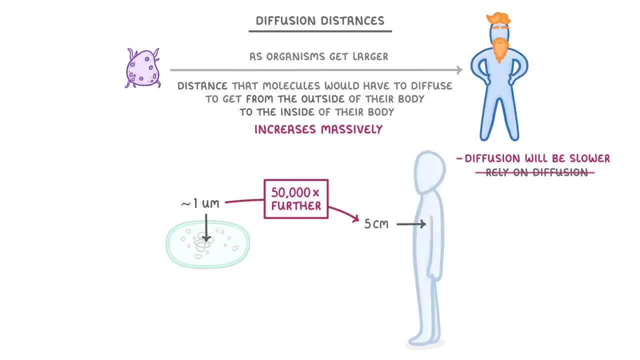 that they need into their cells. To solve this, larger organisms often have transport systems, like the circulatory system, which transport molecules from the exchange surfaces where they enter the body to the body, to whichever cells need them. This means that the molecules then only have to diffuse a very short distance to get into 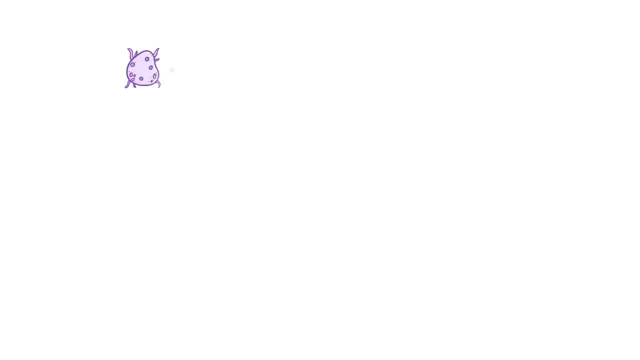 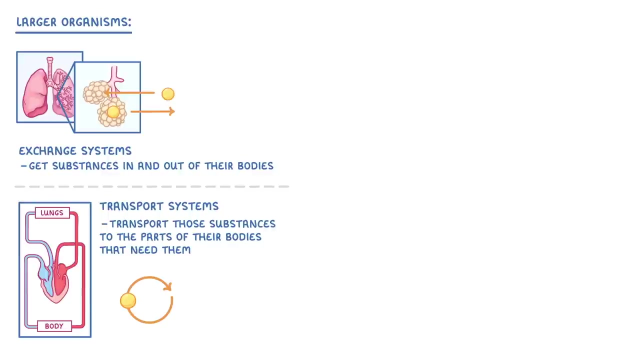 the cells. The takeaway here is that larger organisms generally have exchange surface to get substances in and out of their bodies and also transport systems to transport those substances to the parts of their bodies that need them. same ideas apply to plants, For example. they have roots and leaves to exchange substances.